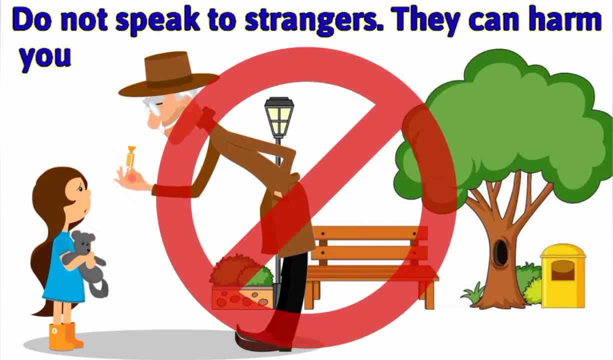 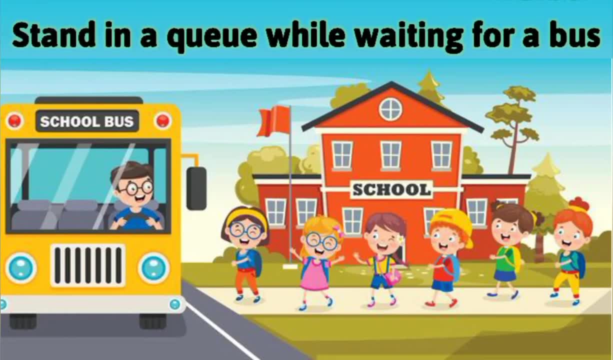 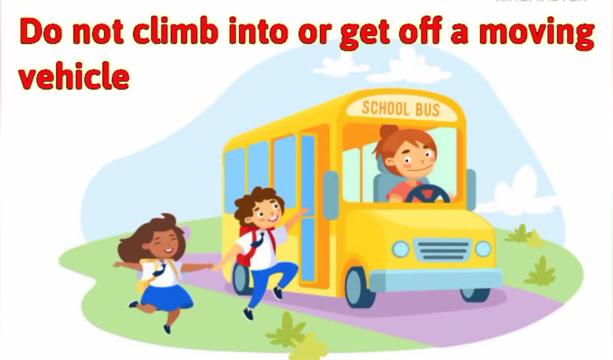 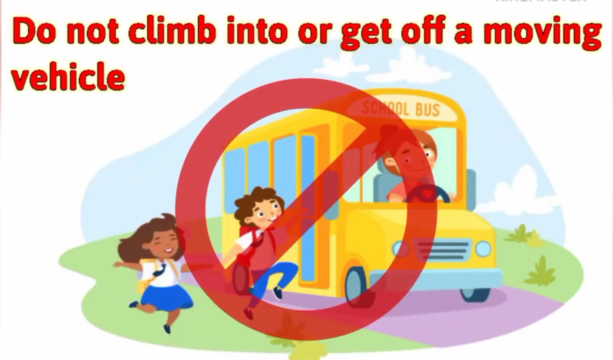 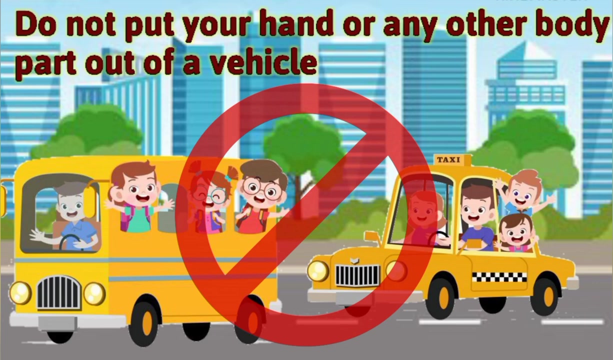 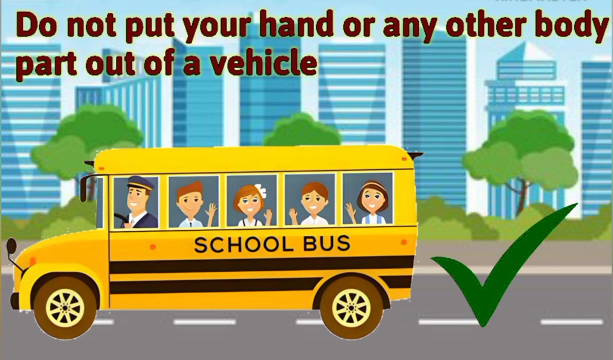 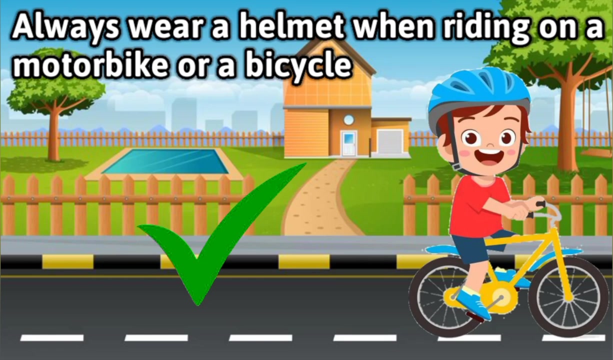 They can harm you Safety while travelling. Stand in a queue while waiting for a bus. Do not climb into or get off a moving vehicle. Do not put your hand or any other body part out of a vehicle. Always wear a helmet when riding on a motor bike or a bicycle. 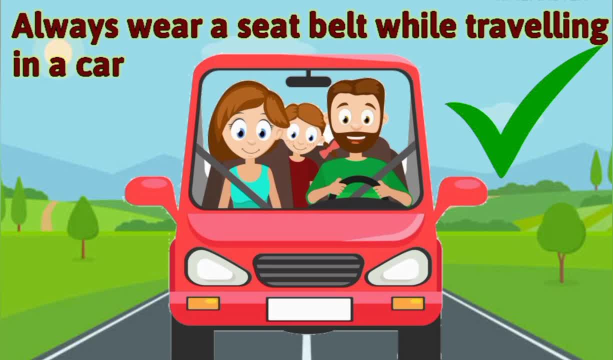 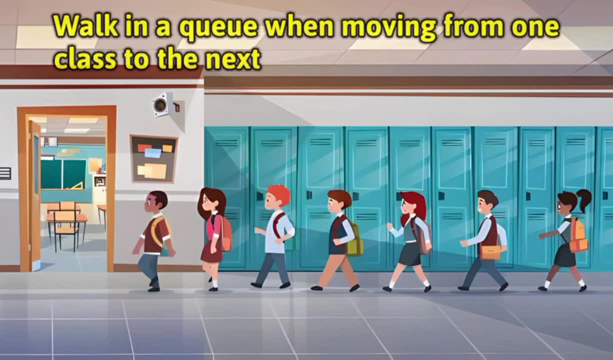 Do not forget to wear a seat belt while travelling in a car. Safety in school. Always walk in a queue when moving from one class to the other. Always wear a seat belt while travelling in a car. Safety in school. Always walk on a queue when moving from one class to the other. 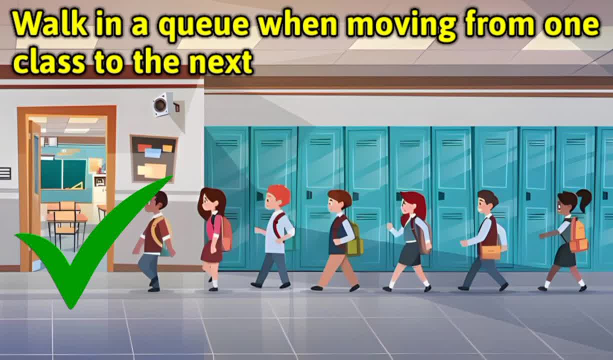 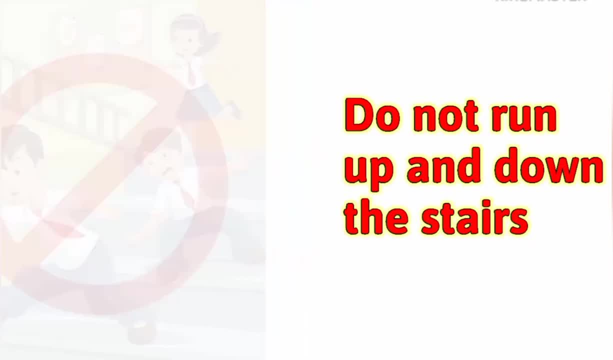 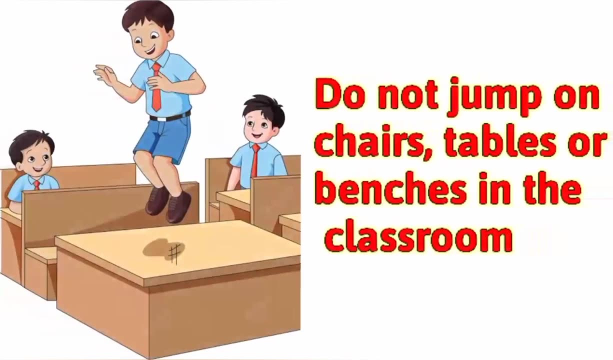 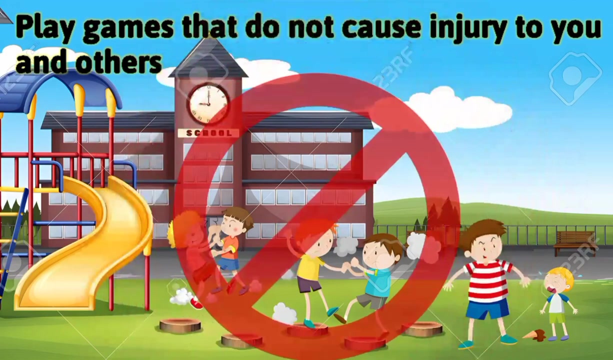 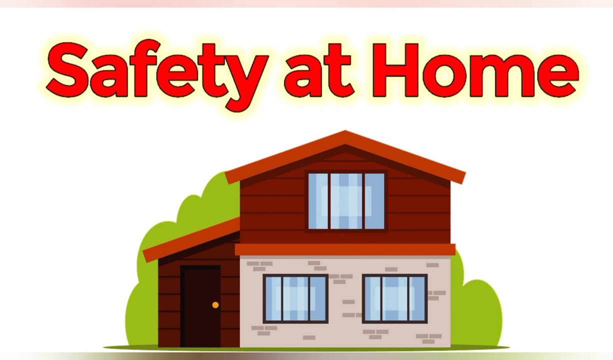 class to the other. Do not roam around in the corridor. Do not run up and down the stairs. You can fall down and get injured. Do not jump on chairs, tables or benches in the classroom. Always play games that do not cause injury to you or others. 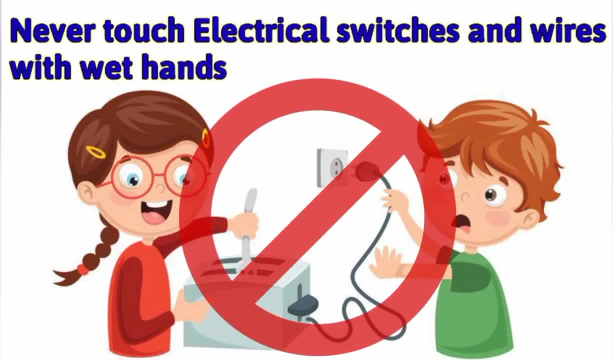 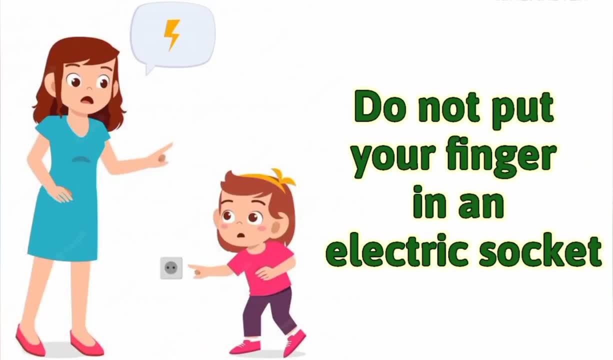 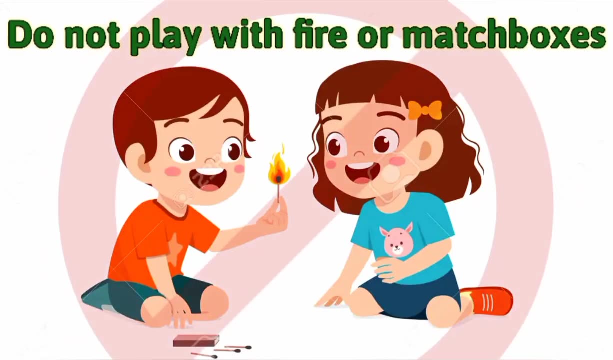 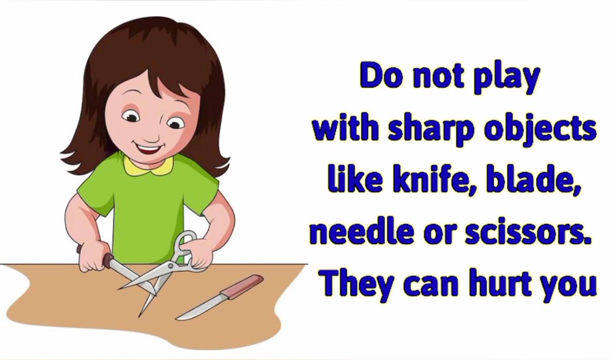 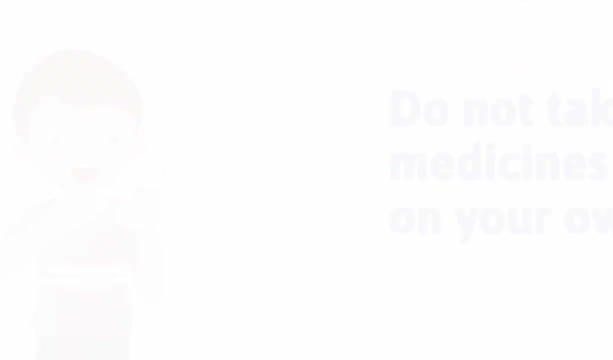 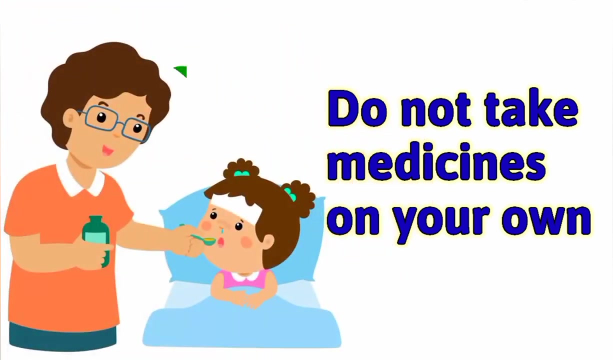 Never touch electrical switches and wires with wet hands. Do not play with toys or animals remotely. situations will cause you injury. Do not put your finger in an electric socket, fire or match boxes. never play with sharp objects like knife, plate needle or scissors. do not take medicines on your own. always take the help of a doctor.